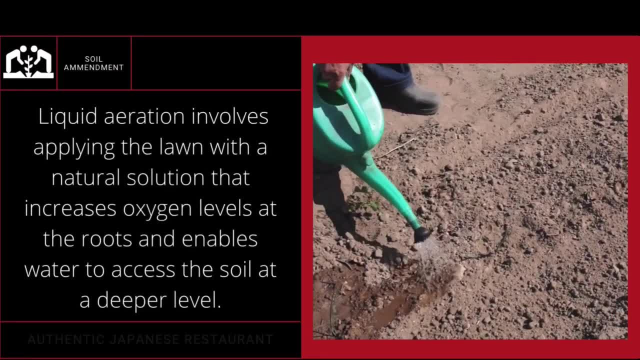 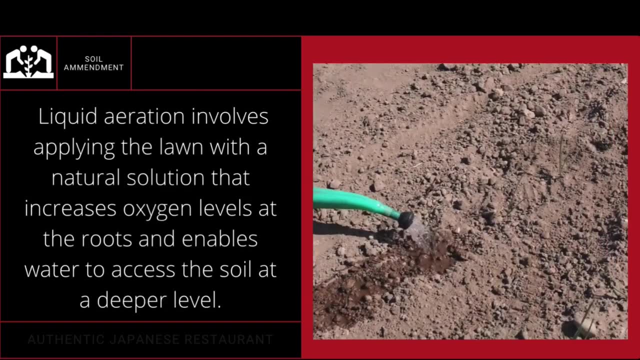 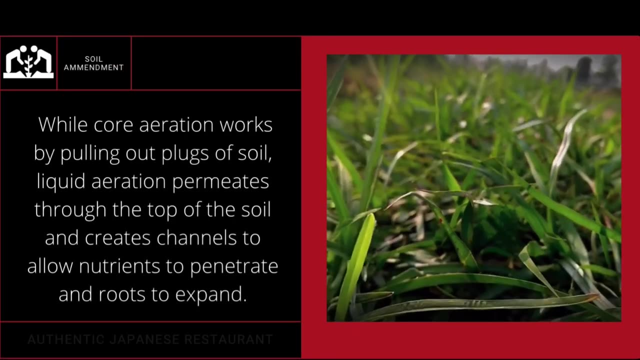 and around this type of commentary. so liquid aeration involves applying the lawn with a natural solution that increases oxygen levels at the roots and enables water to access the soil at a deeper level. while core aeration works by pulling out plugs of soil, liquid aeration permanates. 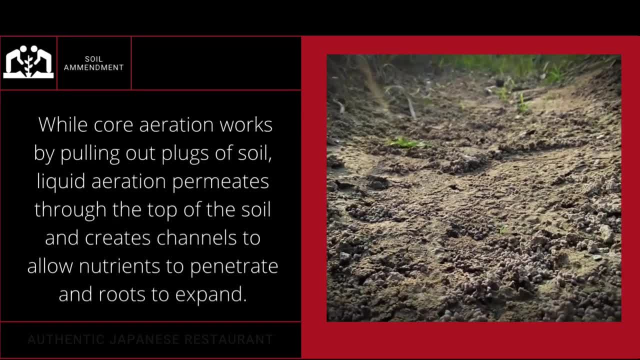 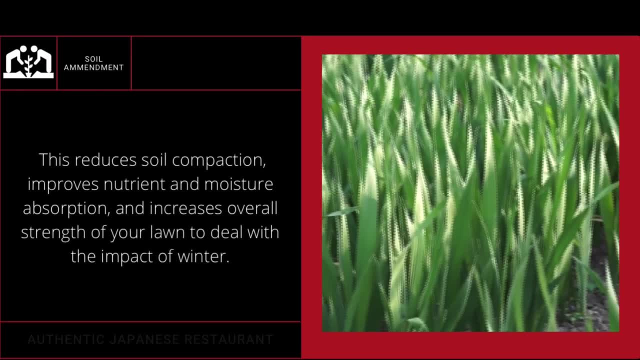 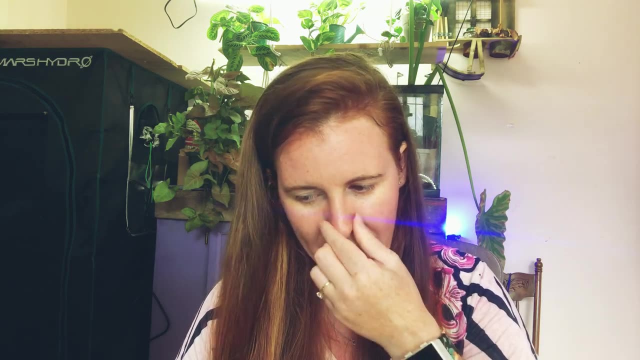 through the top of the soil and creates channels to allow nutrients to penetrate the roots and expand. this reduces soil compaction, improves nutrient and moisture absorption and increases overall strength of your lawn to deal with the impact of winter. so let's dissect this just a little bit. claim is: it works just as well as mechanical aeration. so mechanical aeration? 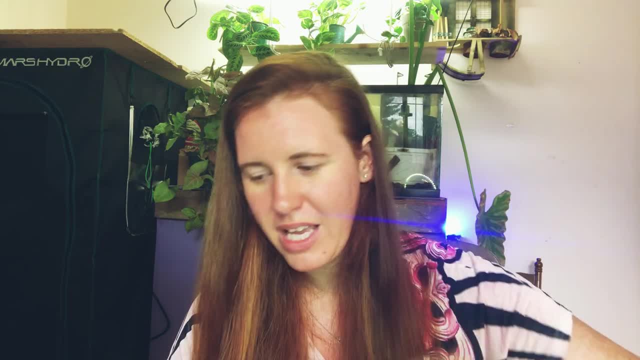 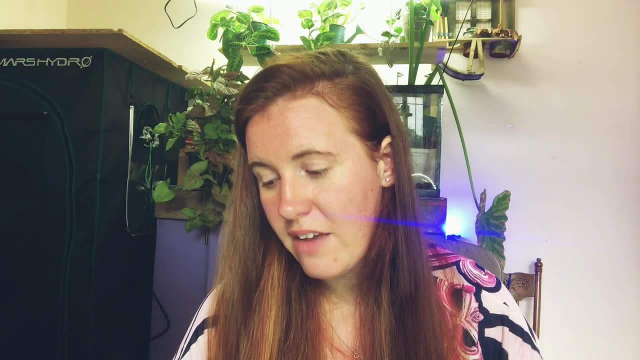 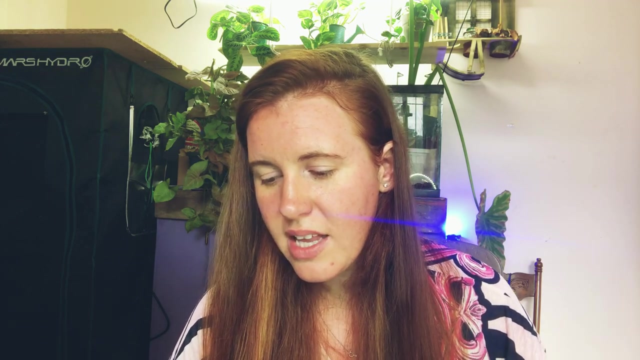 is when you get the little dog doo-doo type looking soil plugs ripped out of your soil, which does work, especially on lawns, and it works very, very well on heavy clay soils and it is a very common way of helping your lawn out. so it claims it is going to do the exact same way as 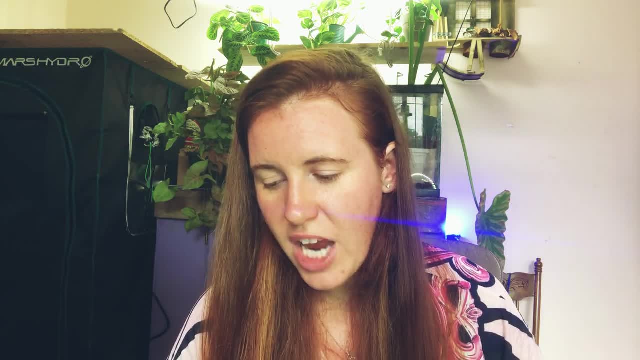 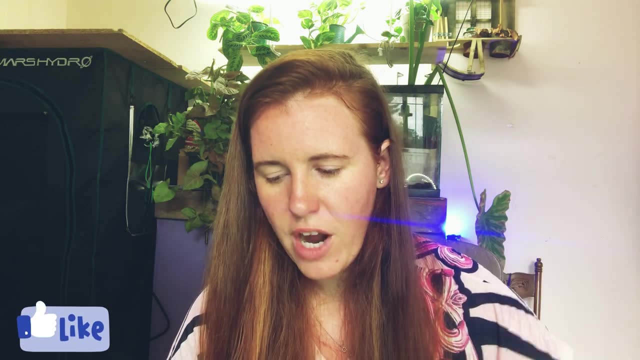 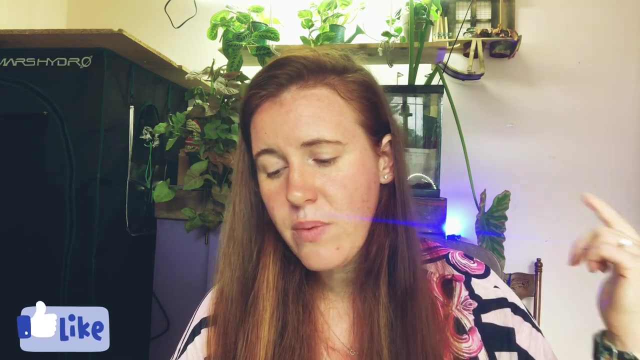 mechanical aeration and it's going to create channels and allow nutrients to penetrate and the roots to expand. so what they are saying right off the bat is telling me that they are either flocculating the soil or they are dispersing the soil. so the only way to look at air, liquid aeration. 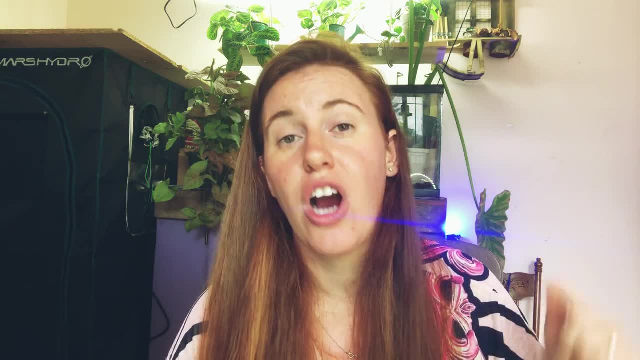 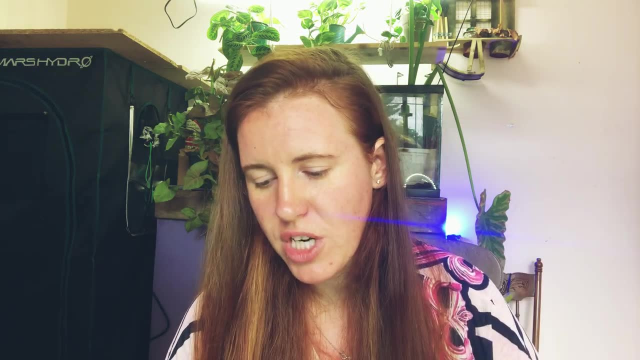 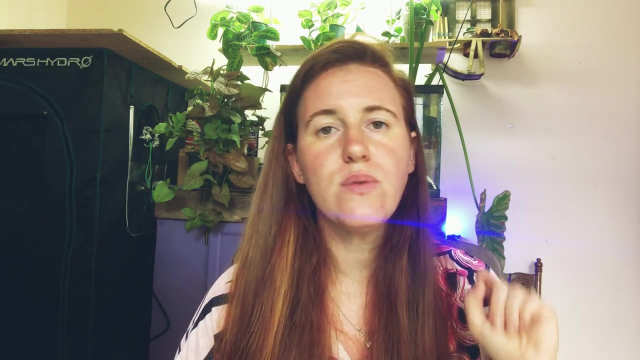 is to determine what chemical is in there and what charge that chemical has, to determine what mechanism they are using within the soil- flocculation or dispersion. so let's first look at what flocculation is and then let's look at what dispersion is. so flocculation is something that happens in clay soils and the effects of 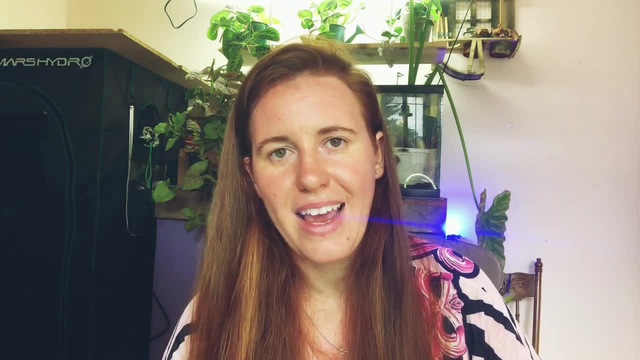 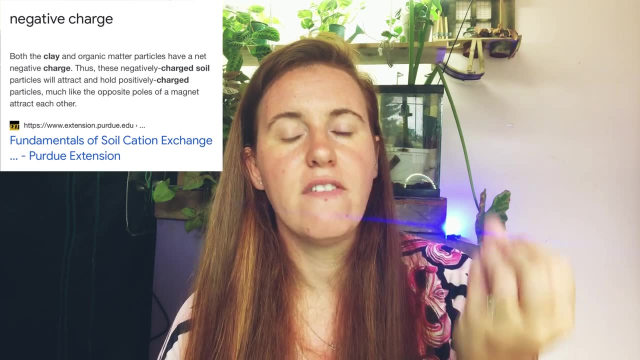 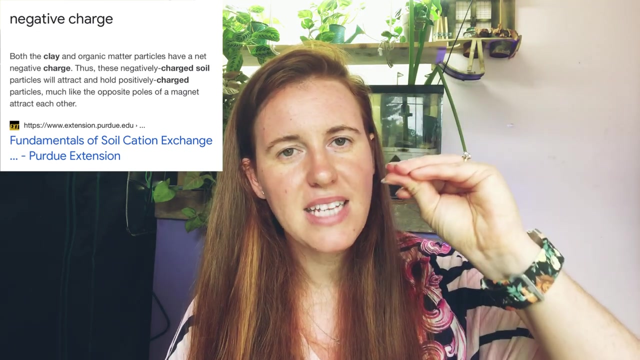 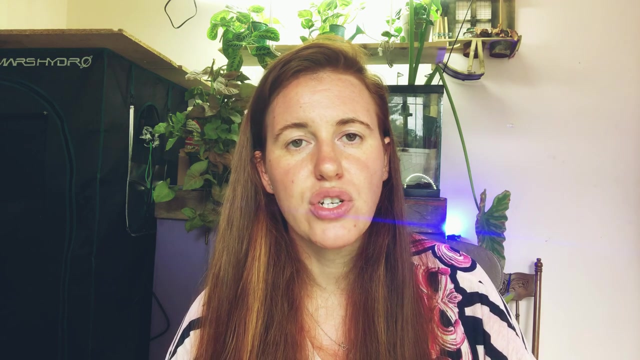 flocculation tend to decrease the lower our cation exchange capacity is. so with cation exchange capacity, our clay soil, our soil is negatively charged, meaning if we add a positively charged ion to it it adds like a magnet and it just glues itself together and it kind of makes these aggregates. and we can see this if we dig out with a soil. 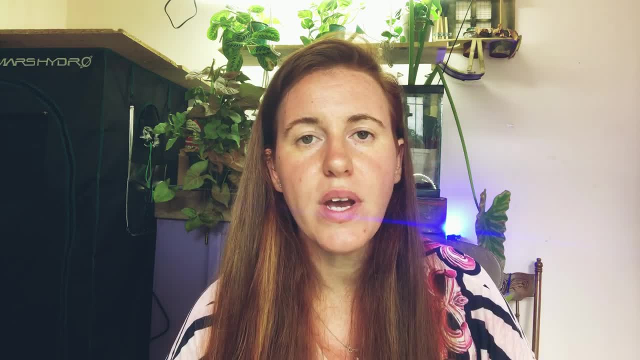 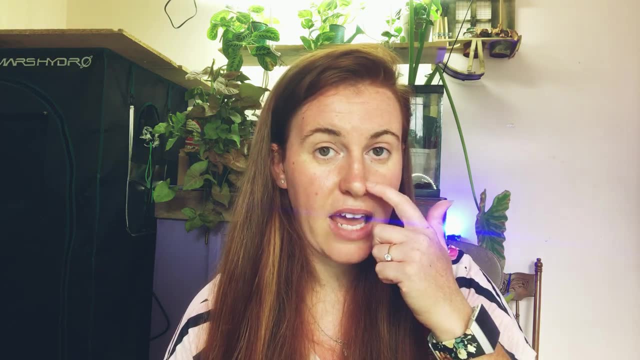 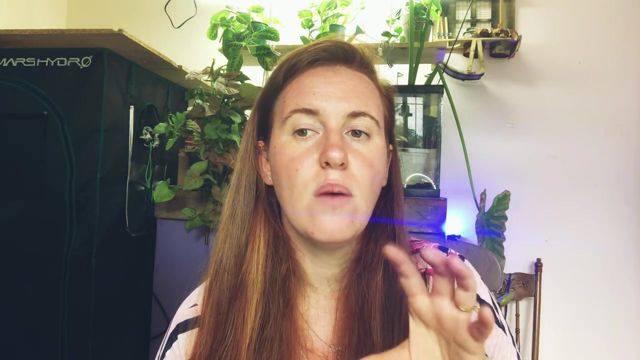 shovel, we will see aggregated clumps of soil and this is a very, very good sign that well, we have flocculation happening. so flocculation is a very good way of um it does I mean cause compaction to an extent, but it helps with structure, meaning if we've rototilled our soil within an inch of its life. 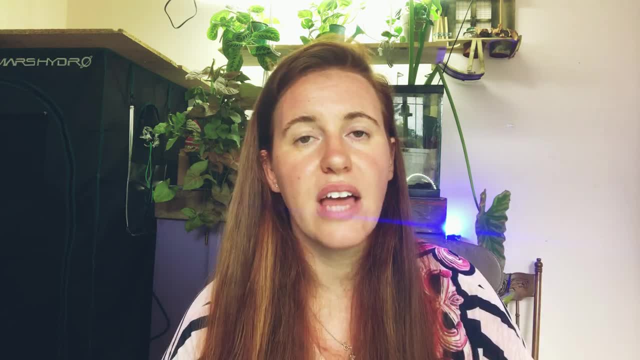 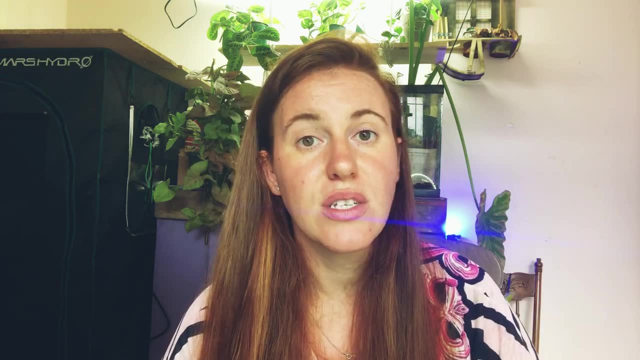 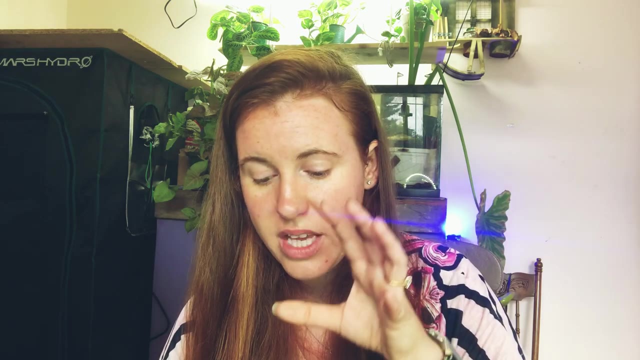 we can use flocculation to help bind that soil together to reduce things such as erosion. so if you have a big erosion issue with your soil, then flocculation is your solution. so we need to add a positively charged uh cation to the soil structure and these can come in the form of calcium potassium. 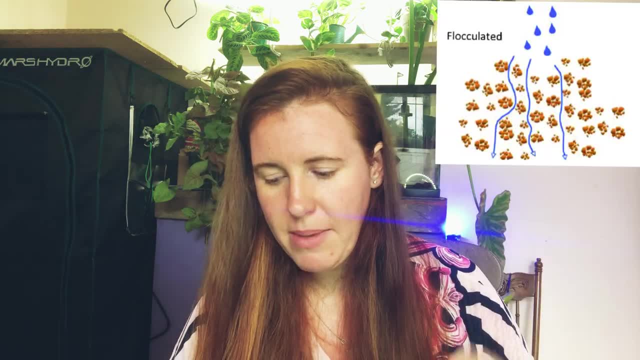 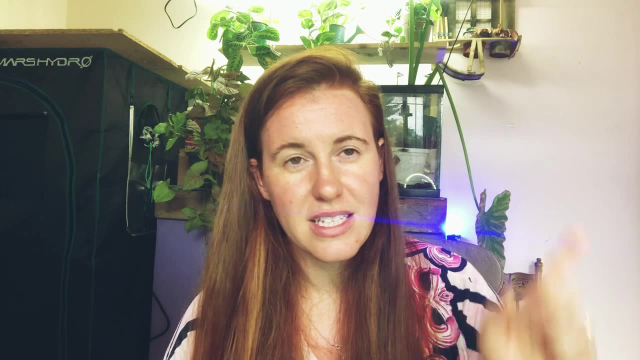 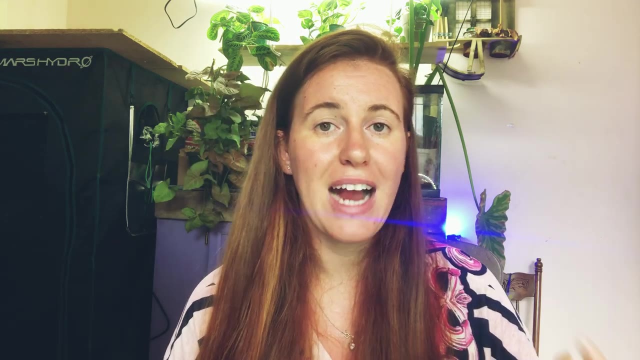 magnesium sodium, you name it. this will cause flocculation and coagulation within the soil structure, and so I don't think that this is what they're doing here, because we have a lot of flocculation happening out in our lawns or in our gardens, especially for adding fertilizer, so fertilizer that contains any. 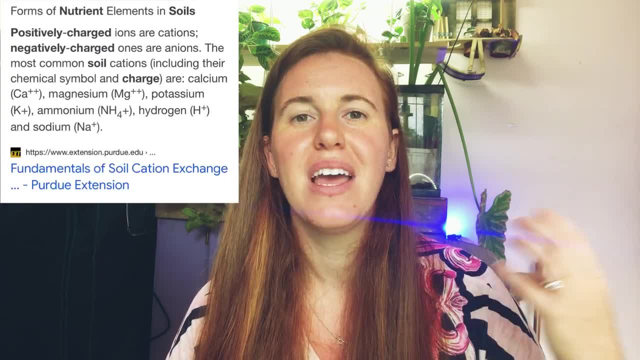 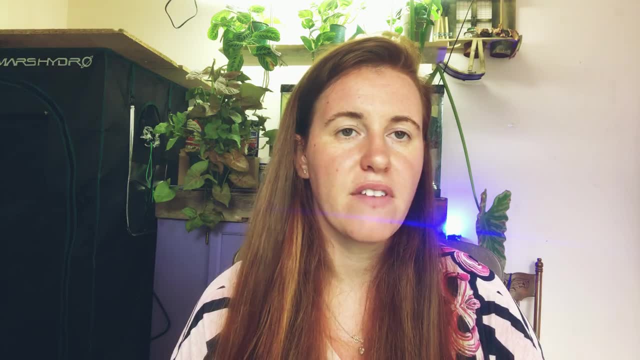 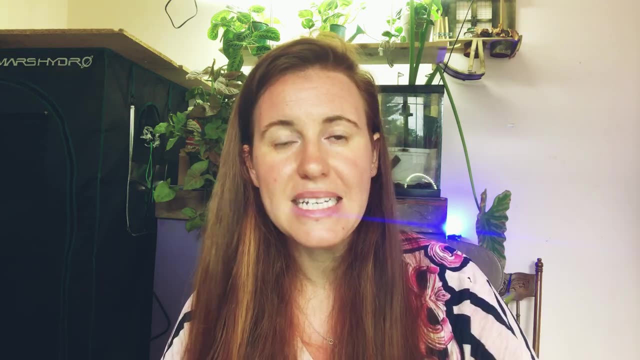 level of sodium, calcium, magnesium, potassium is going to have a positively charged ion and so therefore, so long as we're not rototilling, flocculation is going to be very, very high, which I think the mechanism they are using is actually dispersion. so dispersion is the absolute opposite. 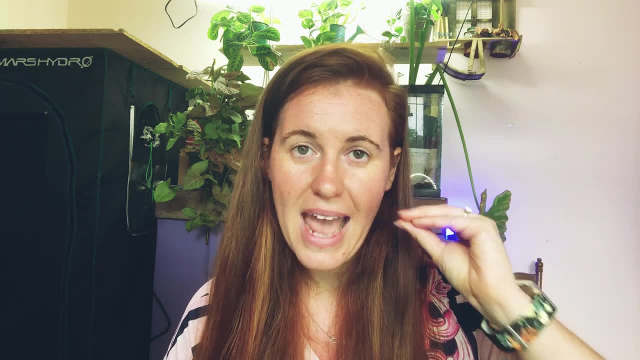 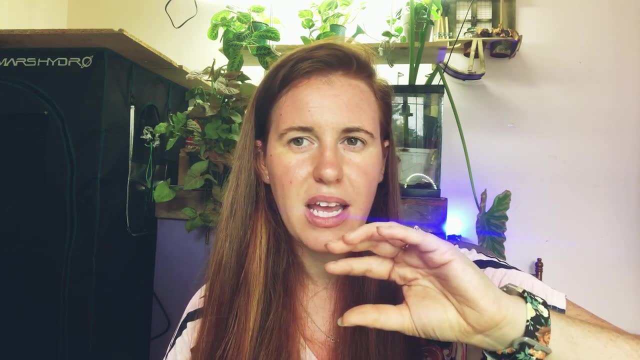 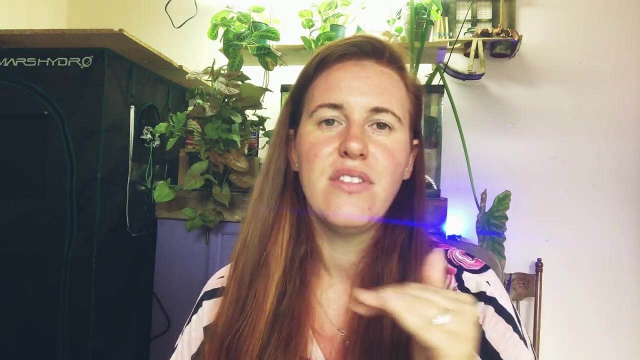 of flocculation and so it's actually going to use a negative, an ion, to repel the soil from each other. so it's going to bind with the soil, um, and not in the way that flocculation will. it will kind of- you know, anti-gravity- for lack of a better term- the soil and help keep things really light and fluffy. 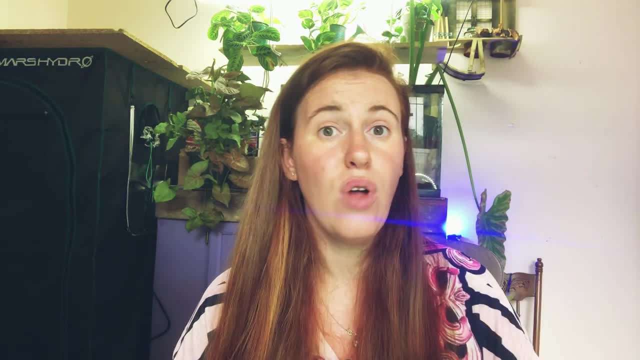 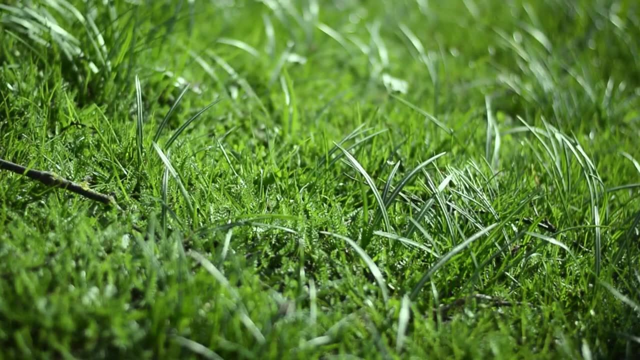 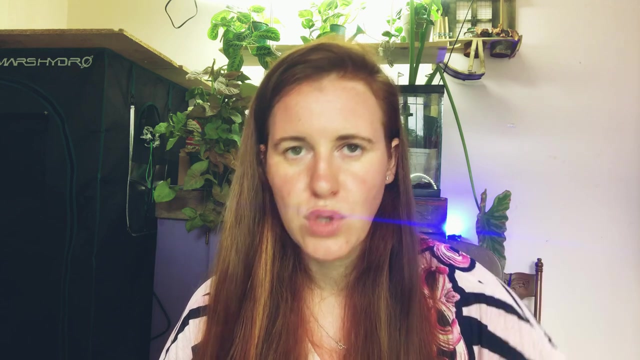 which is what we want in the case of our soil, uh, in our lawn, because the pressure of human activity- lawnmowers, vehicles, snow, the lack of rototilling, the very you know, the roots of our grass don't really penetrate very deeply because we usually don't use fescue, we use things like Kentucky bluegrass on our lawns, and so we have. 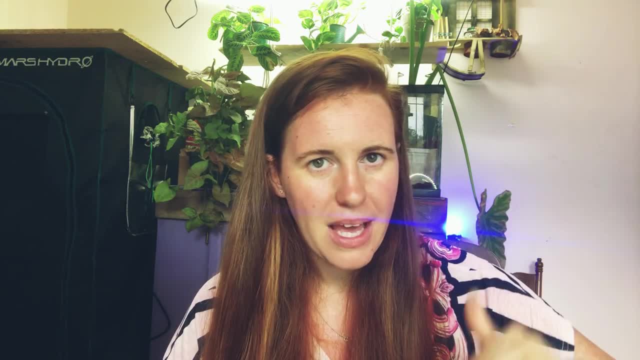 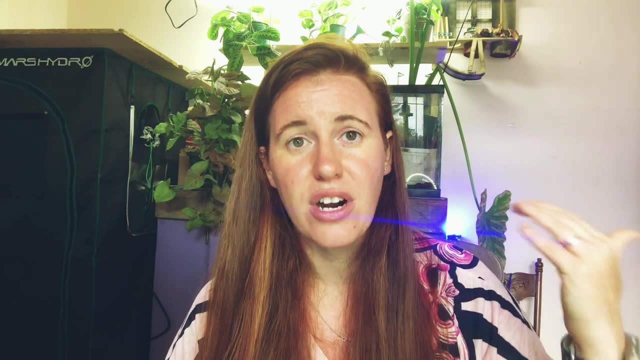 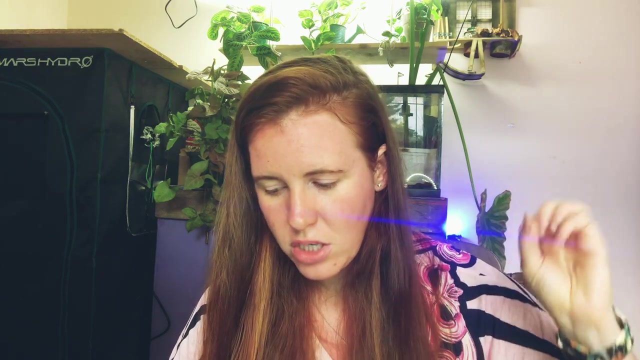 a very subsurface type root system that doesn't penetrate down. we don't have any tap roots or anything crazy like that, so flocculation and compaction is a definite issue within our lawn structures. however, dispersion is going to force everything to pop apart, for lack of a better term which will help with water infiltrate, infiltration, nutrient. 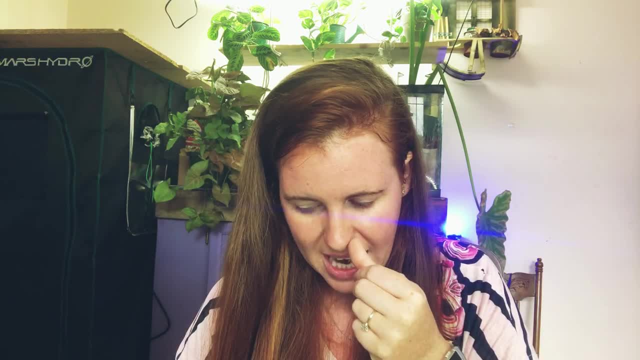 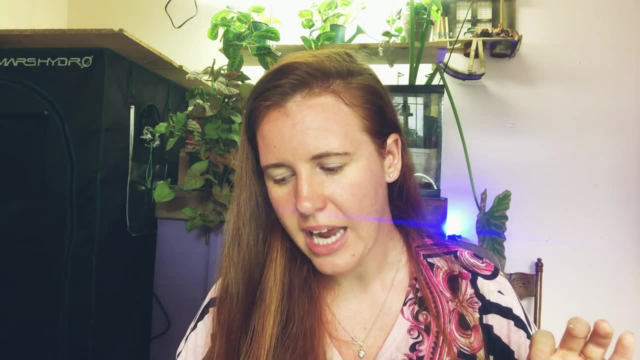 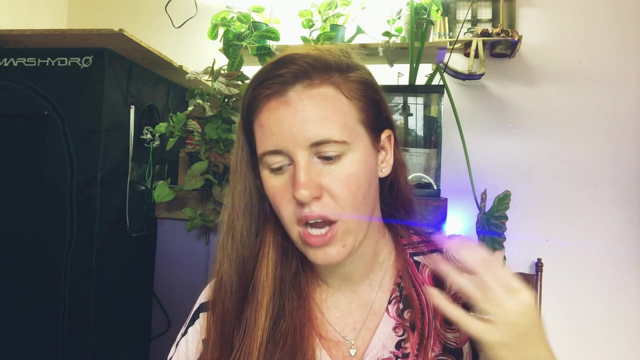 capture and root penetration is all going to happen here in this case. now, when you look online- I don't know why- I usually what I do with these videos is: I will look in the journals that I have access to through my university log in. I will look at the scientific journals. then I also Google what you guys are seeing. so 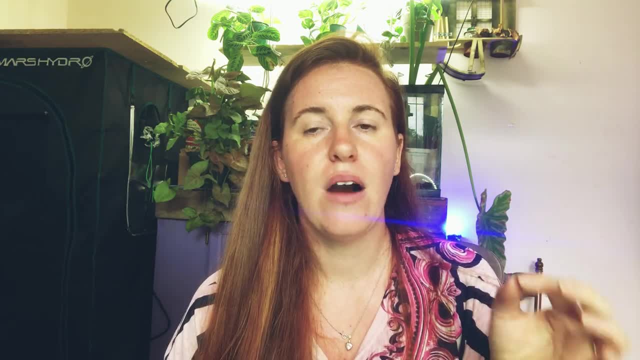 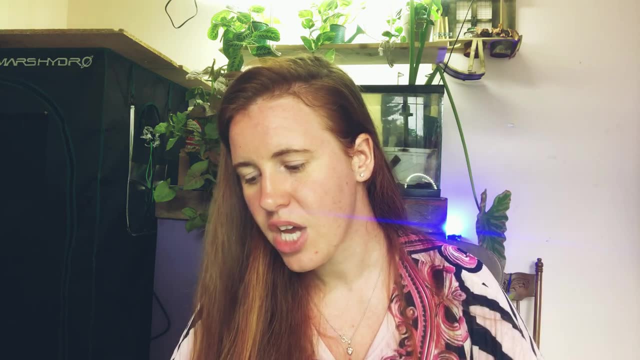 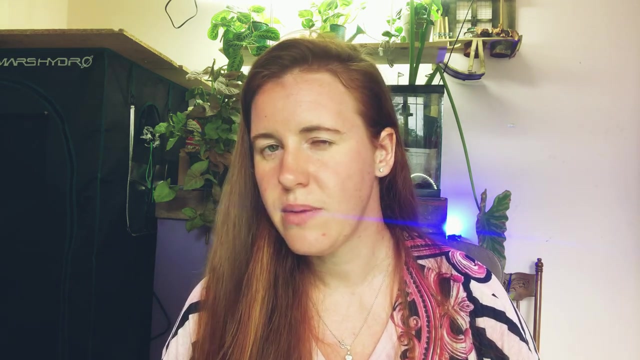 I will Google, for example: um, how does dispersion work in soil? because I want to see what the common answer is that you guys would see without the science attached. and so a lot of bloggers and influence out there are saying that sodium can cause dispersion. sodium doesn't cause dispersion. 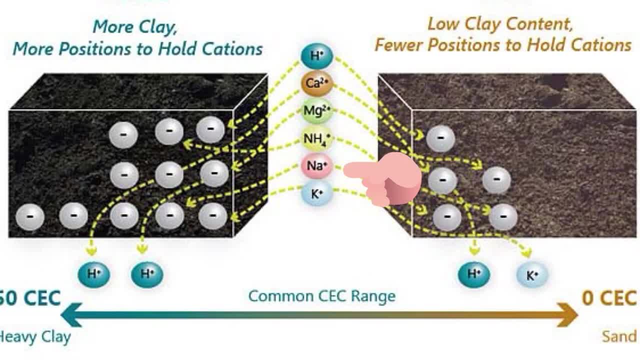 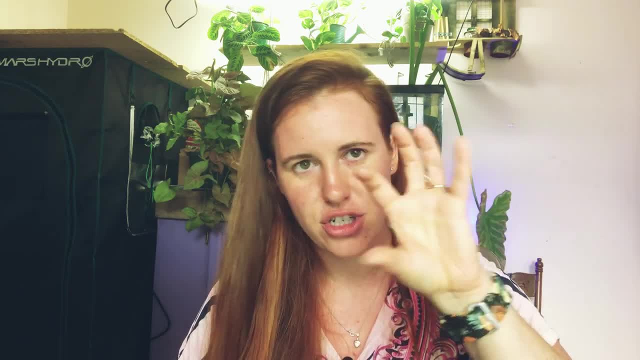 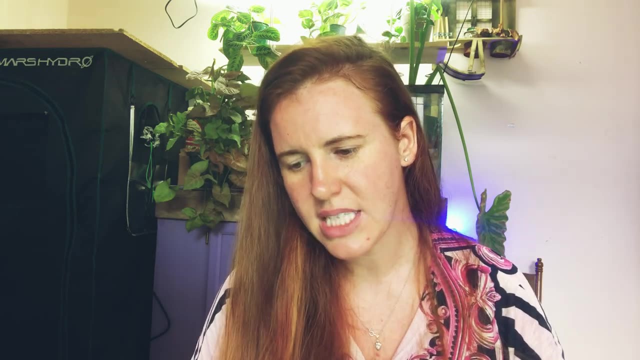 sodium has an na plus one, so the plus one is enough of a plus plus. it's going to cause flocculation, so it's going to cause compaction and um aggregation within the soil. so I don't know why a lot of sites are saying that. but that's, that's false. 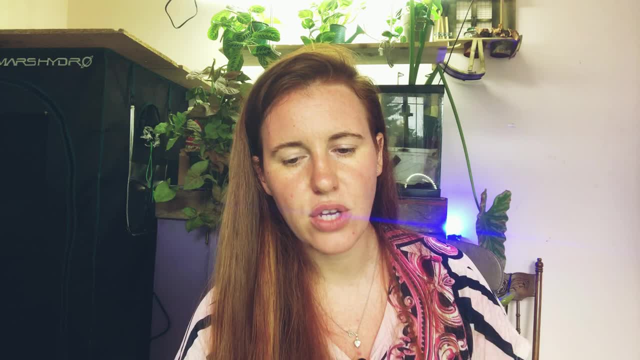 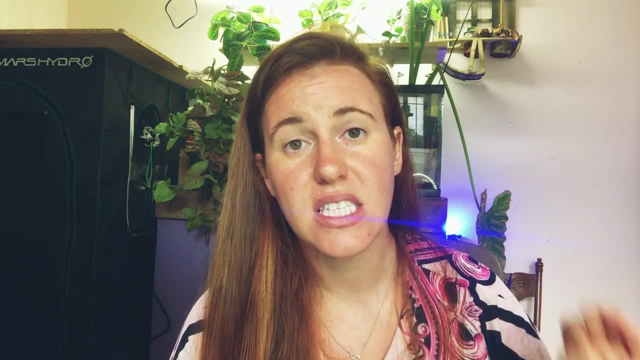 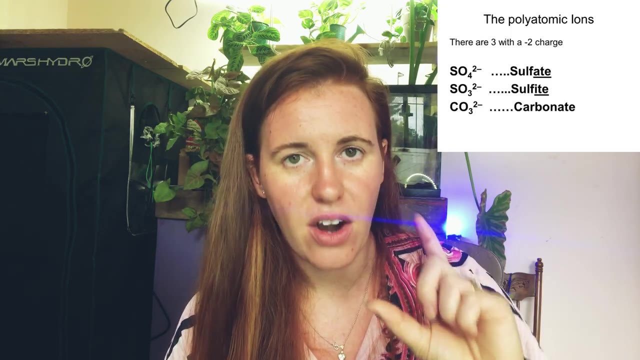 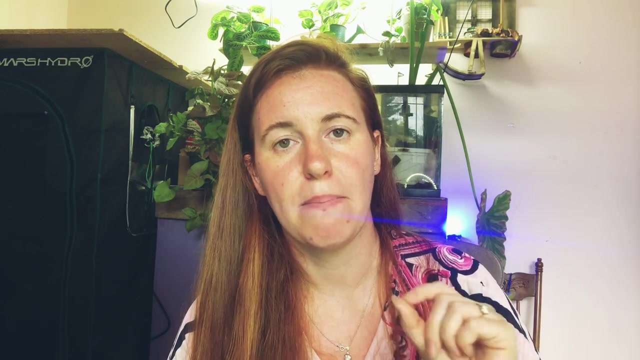 so don't listen to that. I'm not lying to you. I promise you need a negative charge. so nitrates, nitrites will cause this. phosphates, sulfates, so, um, all are versions of nutrient profiles that are by plants or in are in the proper form for plant uptake and they have negative charges to them. 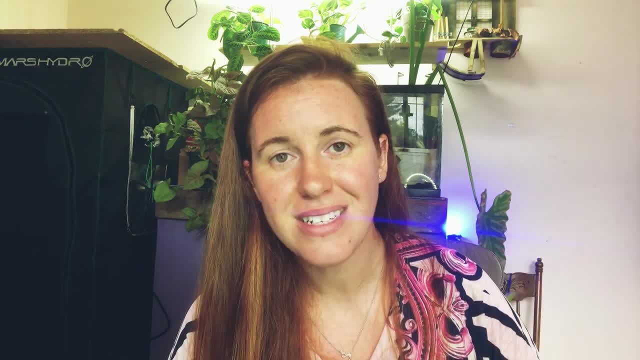 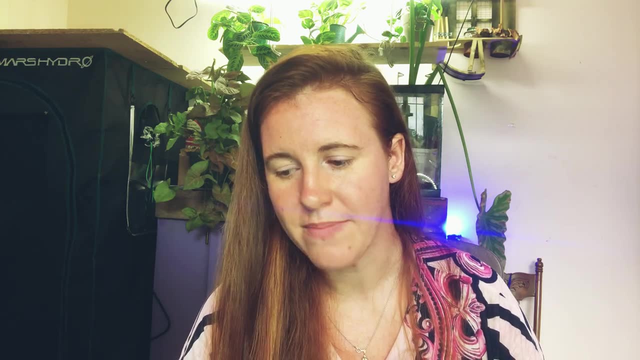 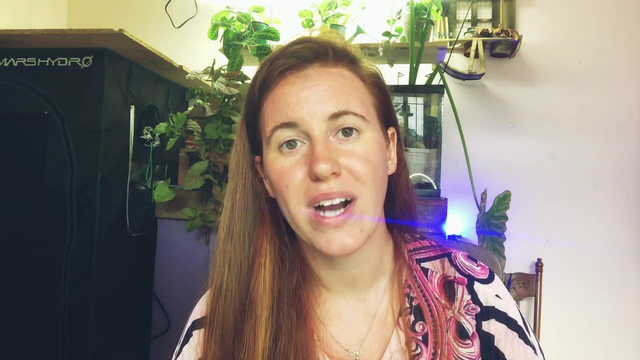 meaning they will push things apart. so it can have a negative one, you can have a negative four, it doesn't matter, so long as it's negative, it's going to cause dispersion in some way. so this is where it gets a little bit murky. it's very difficult for me to say what is in every single. 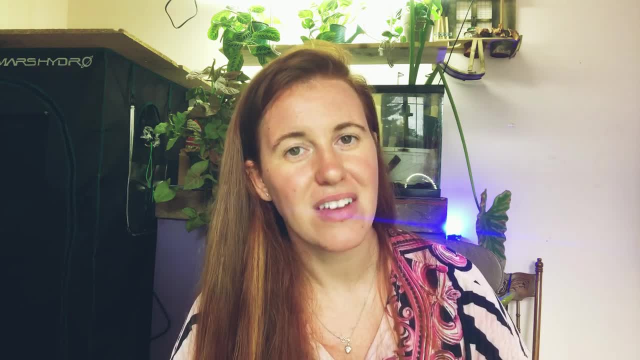 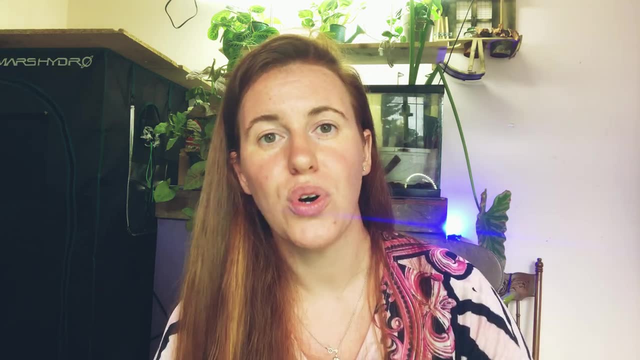 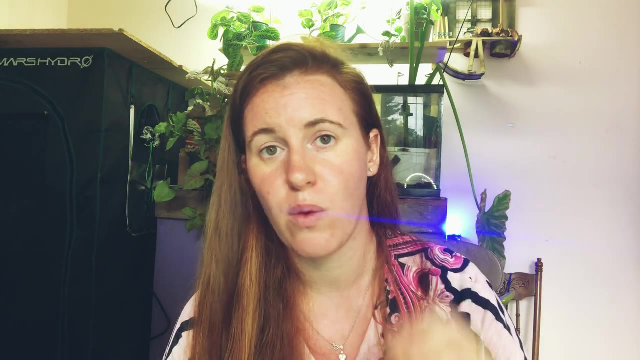 liquid aeration product. they all seem to have a slightly different montage of what's in there, but I will leave some Amazon links down below for actual negatively charged compounds, active ingredients within the liquid aeration that will cause dispersion and will not cause flocculation, because again, we want dispersion, we do not want flocculation in this case. 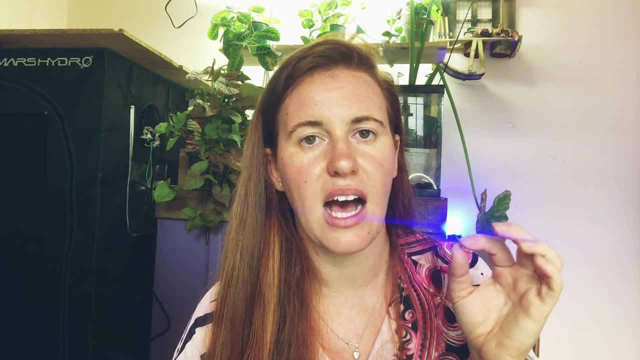 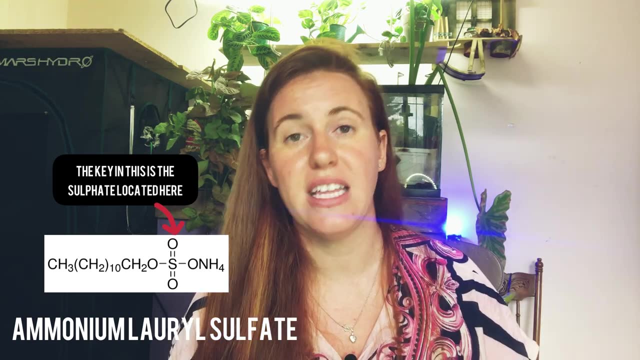 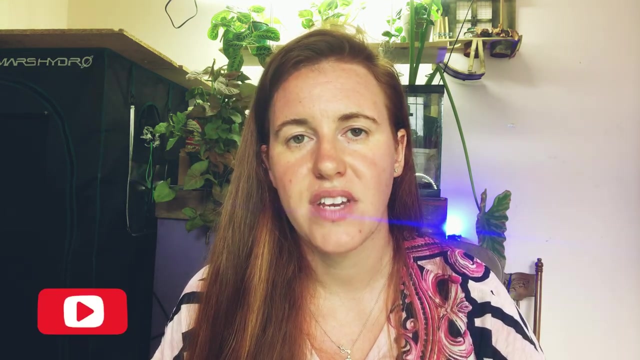 the most common compound active agreement is ammonium laterite sulfate, which is negatively charged and therefore will cause that dispersion and therefore will be a very successful version of liquid aeration. now I can't guarantee they all have an active ingredient with a negative charge, so the easiest way to figure this out- if you are at the 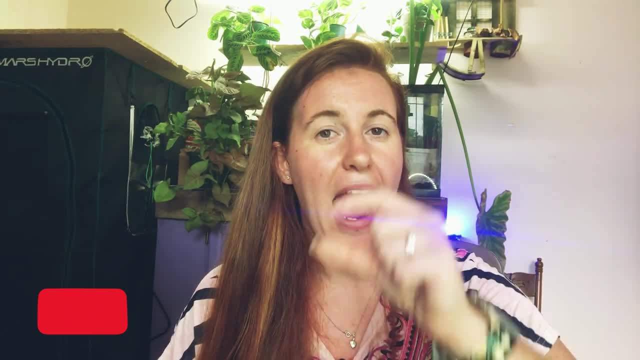 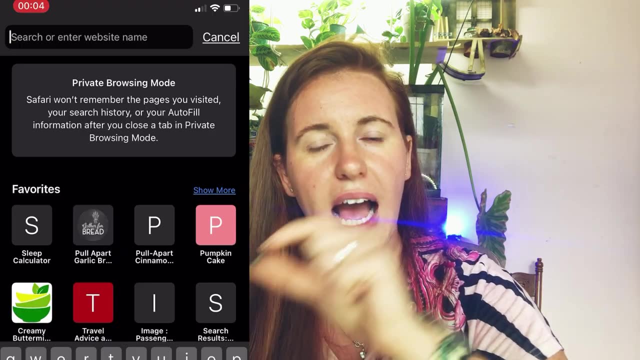 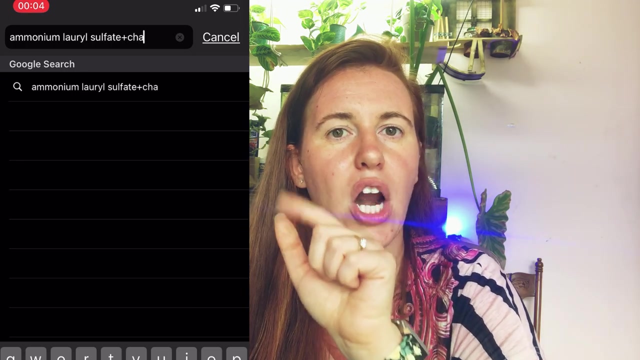 store and you don't want to use the Amazon links before if you want to look at the active ingredients list and you want to type in the name of the active ingredient into Google and then you want to say, uh, put a plus sign and say, um, Ionic charge. 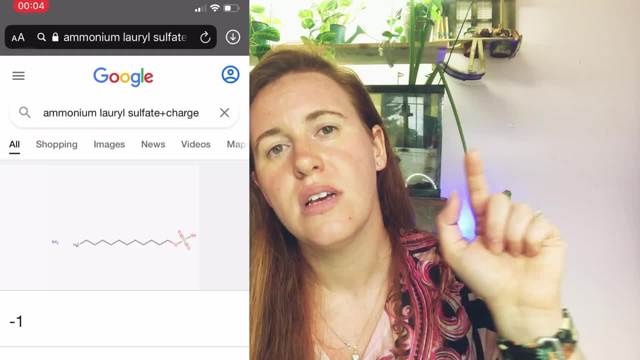 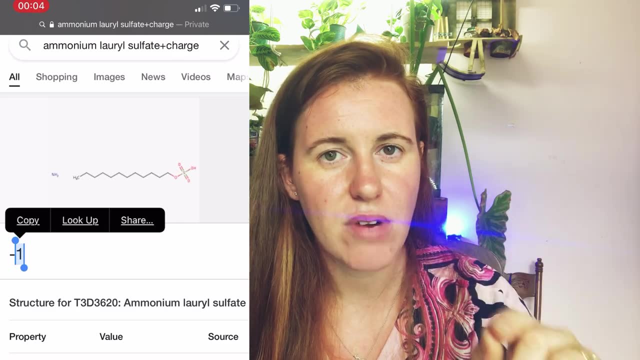 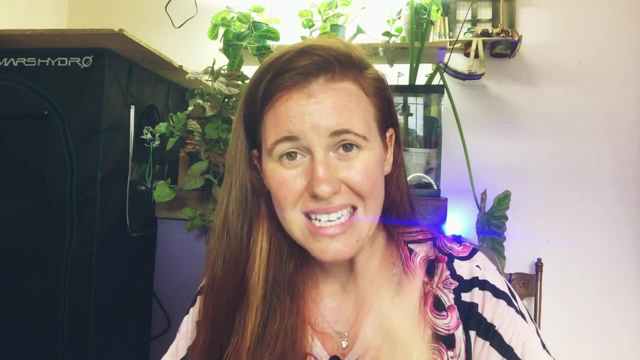 so Ionic charge, and Google, oddly enough, is very good at telling you what that charge will be. so long as it has a negative number, it does not have a zero and it does not have a positive number, you are okay, and that product will work just fine for you. now, if you're still not sure, 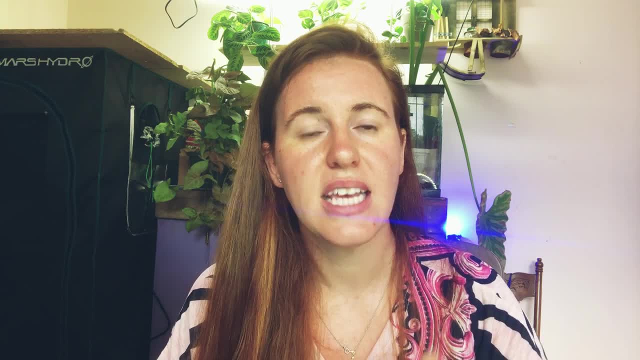 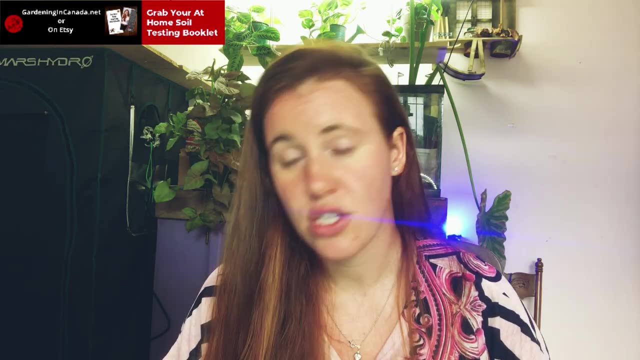 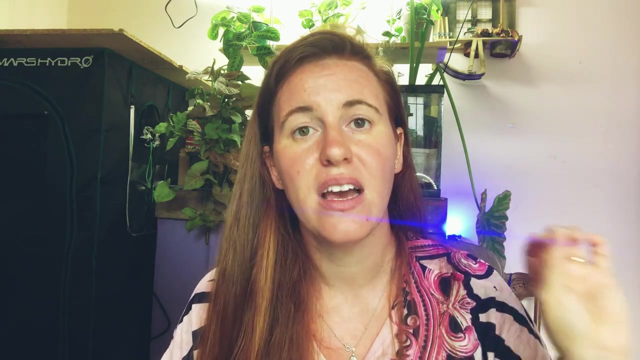 feel free to send me a message gardening canadanet um on the website, on Instagram, Facebook, in the comment section down below, and I will it for you and i will let you know if it's good or not. but overall i do think this product would work. it is working on very basic soil chemistry and, uh, i mean it's gonna work. it's gonna work. 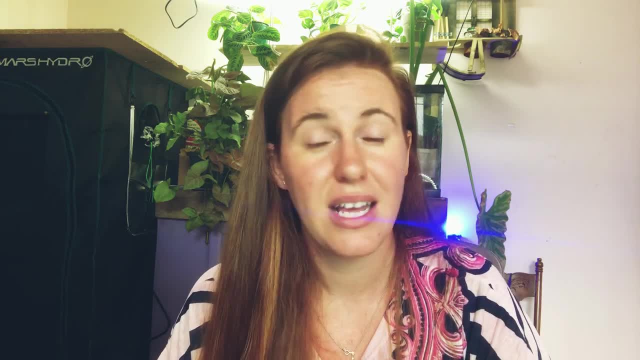 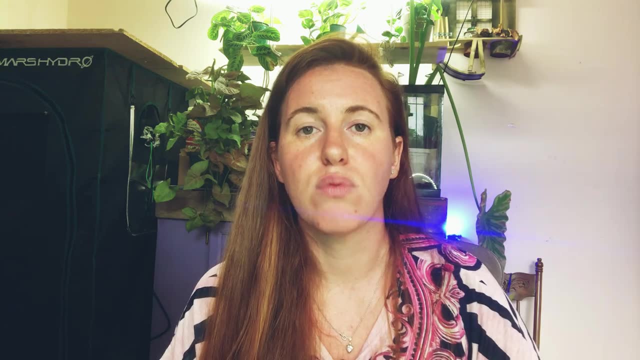 for sure it's going to work. now, is it going to work as good as mechanical aeration? no, it's not going to the liquid aeration. you would have to apply over time, over and over again to see the results of this and the benefits of this. it's not going to be a single application and voila you. 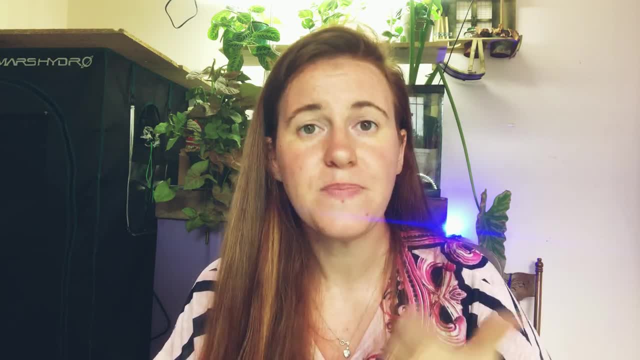 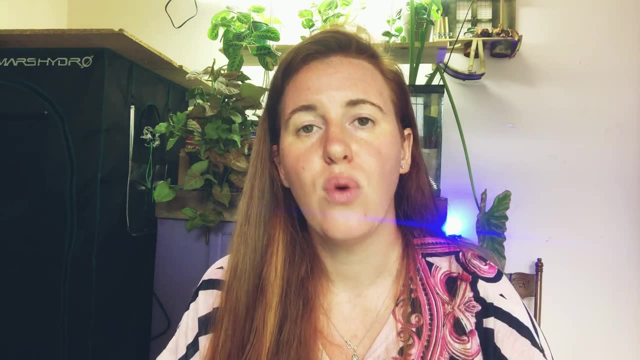 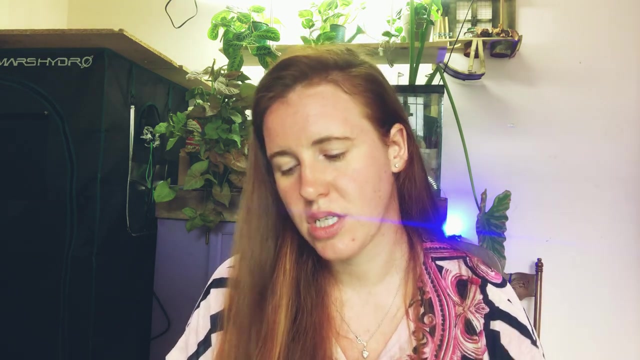 have aerated, so mechanical is going to work much quicker and you're going to have to do it more often. but if you start with a liquid aeration program, over time your soil will disperse and disperse more and more and more so over the years, um, over the season even, you're going to start to